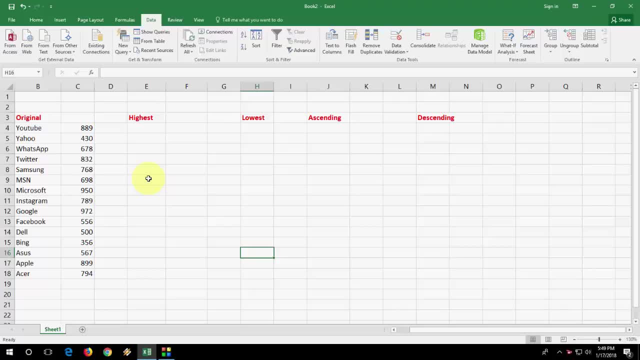 or you can sort highest or lowest value. I'll show the simple way. okay, So when you try to sort any data or value, the common- many people do the common mistake: they select the both data and value and they try to sort like this And this will not work, Believe me. this will not work when 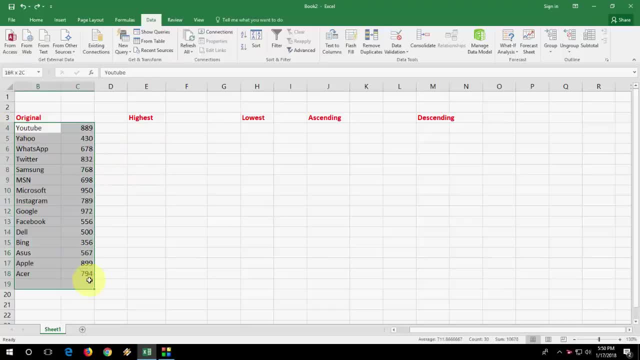 you select the both option. So for this let me copy and paste this one. So here I want to take the highest value along with the data. So don't select the data and value together. Look at that. Just select the value When you're going to. 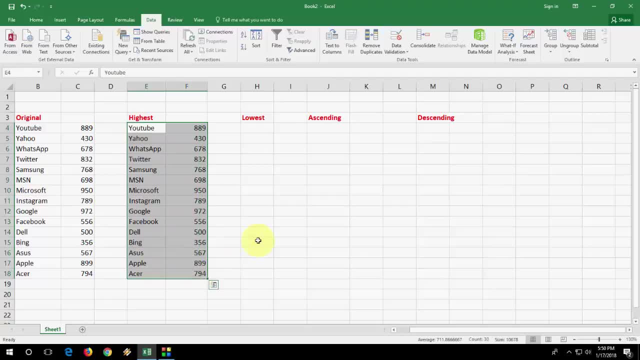 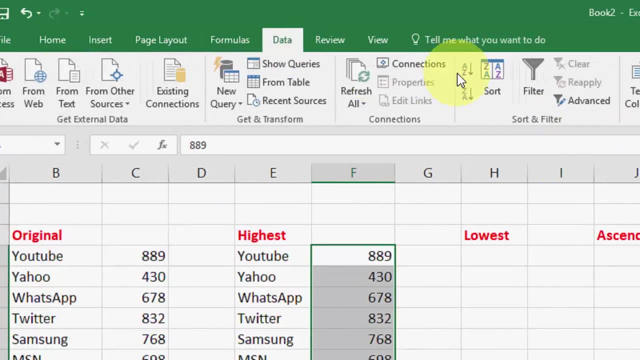 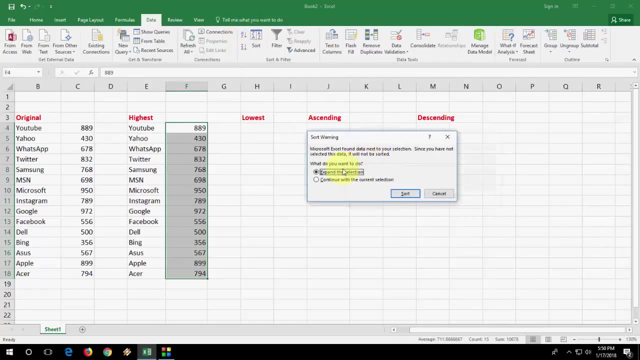 highest value to lowest value. you don't need to select the data along with value, only select the value like this, And then simply go to data here and then you can sort like assigning or deciding, or lower to higher. Click here and you will get the option Like: do you want to? 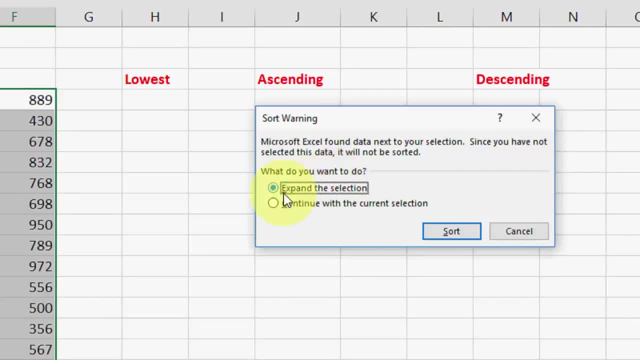 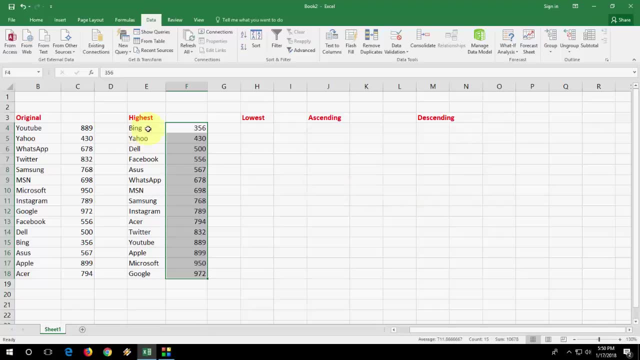 what do? what do you want to do like this: Expand the selection You need to check on. it's an auto default check on, So check on, expand the selection and then sort And boom. as you can see here, Bing is the lowest with alphabetical order. Look at: 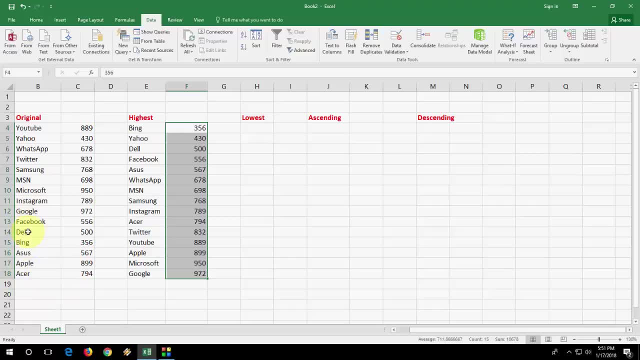 Bing is the lowest here. And then, if you want to highest value, first click here and then sort. this is the highest value. So this is it is clear How to sort this: Highest to Lowest and Lowest to Highest. The same thing here. Copy and paste. I will show the Lowest. 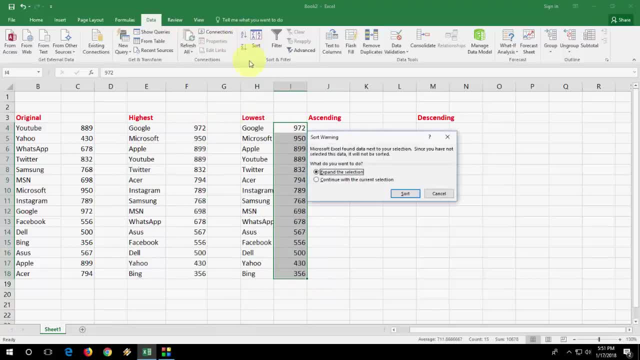 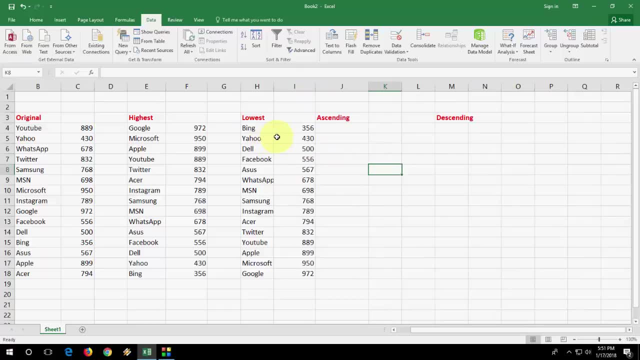 This is the Highest and Lowest. for Lowest, Select it and sort it. So this is the Lowest. Now the Ascending, How to do Ascending or Descending. So if you want to do the Ascending and Descending order, So let me copy this and here paste it. 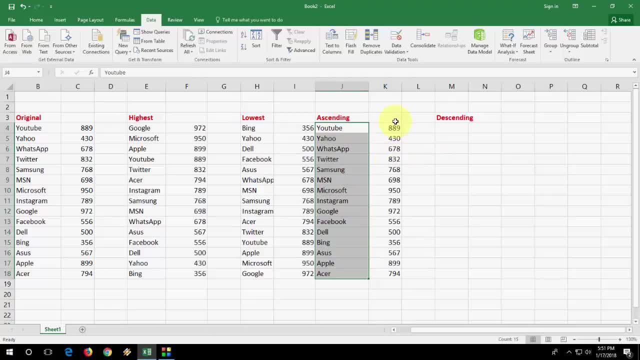 And this time you need to select the data, not the value, because we are going to sort alphabetically, Not going to sort the data. So we need to select the data and it will also affect your value. So now select your data. and now click on Ascending or Descending and click Expanded Sort. 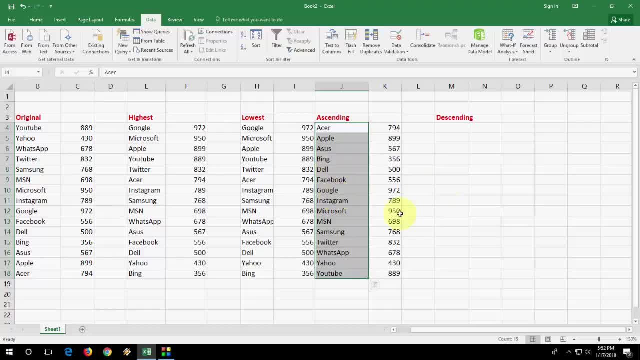 Oh, that's it Simple. Now you can see Apple has come in the Ascending order. The same thing. You can go with the Descending order. So select your only value, not data, Only data, not value, And then click on Descending order And boom, That's it. 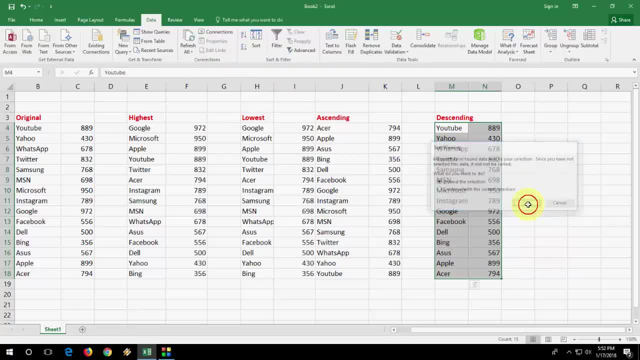 As you can see, YouTube, Yahoo, WhatsApp, Twitter, Samsung Like this. So this is the way. This is the proper way to sort your alphabetically and sort Highest to Lowest or Lowest to Highest. That's it, And one more option. 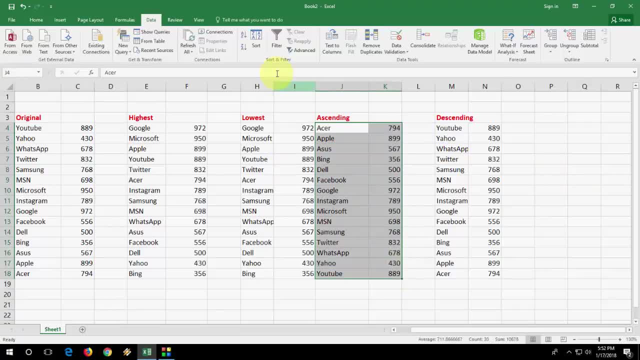 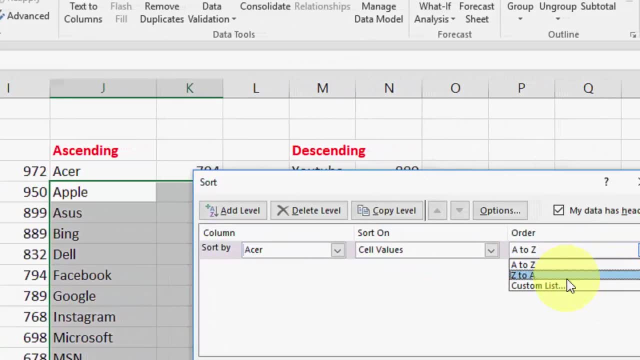 If you want to do some productivity, you can select the value from here and then go to sort, And here you can choose what to sort, Like this, And then you can go with the A to Z or Z to 8. Simple. 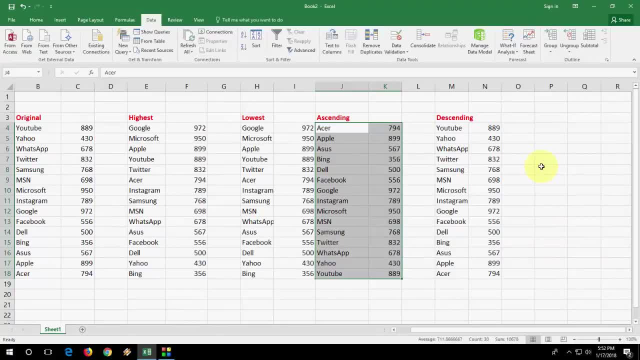 So I hope this video helped you. Thank you for watching. If you have any questions or ask me any comments, please like share and subscribe. Thank you very much, guys. 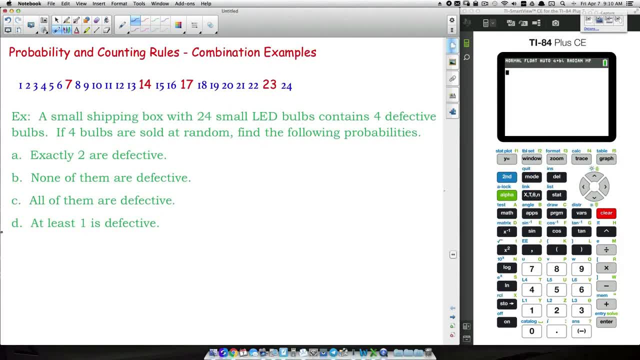 All right, in this video we're going to look at four examples that involve probability and counting rules. These four examples, we will be dealing with combinations and I'm going to you know, stress that to you- Why is this going to be a combination versus a permutation before? 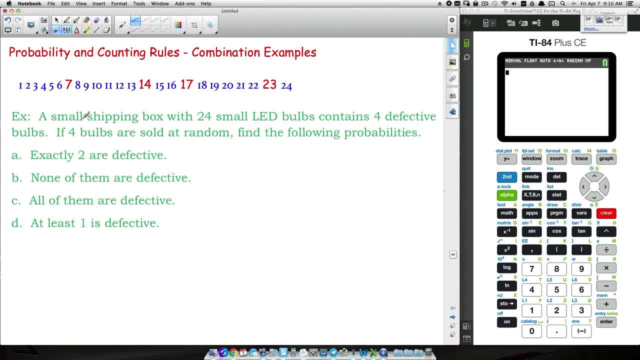 we actually dive into these four examples here. Well, let's look at what we have. A small shipping box with 24 small LED bulbs contains four defective bulbs. If four bulbs are sold at random, find the following probabilities: So what we want to do here is first of all, think about 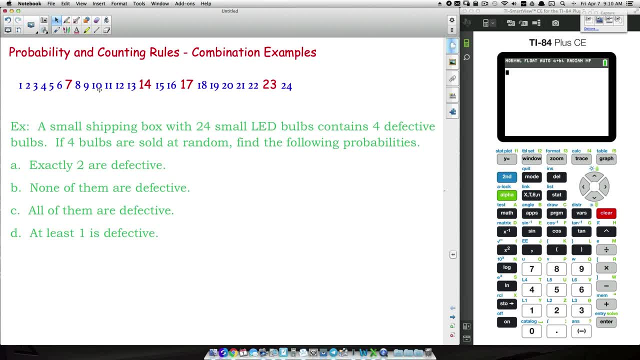 do we have a permutation? Do we have a combination? Which is it? Well, you know, up here I have the numbers 1 through 24 listed. Let's just let these represent the bulbs. So we got 24 bulbs. I'm calling it bulb 1,, bulb 2,, bulb 3, etc. And then, out of these 24, I have